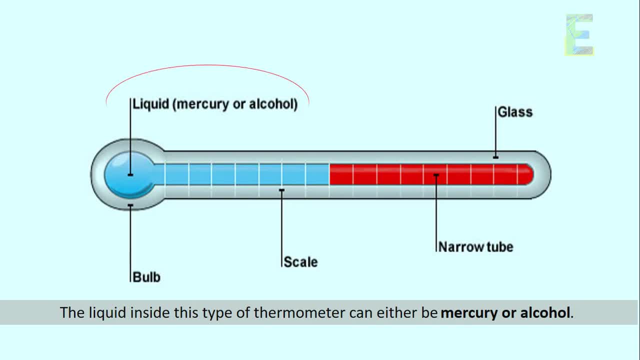 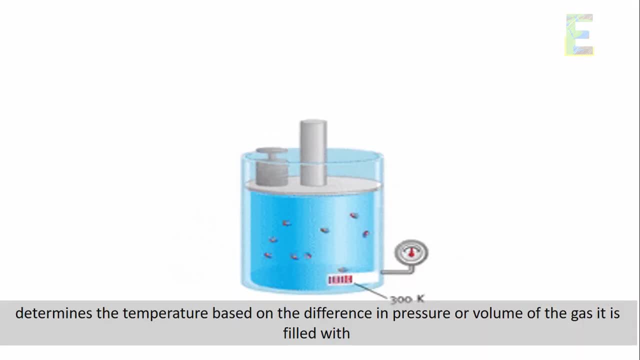 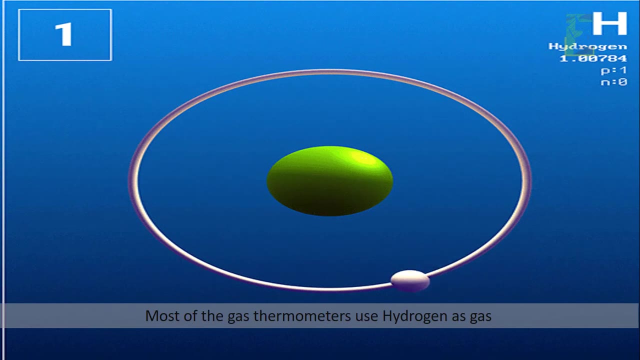 The liquid inside this type of thermometer can either be mercury or alcohol. Next is the gas thermometer. It determines the temperature based on the difference in pressure or volume of the gas it is filled with. Most of the gas thermometers use hydrogen as gas. 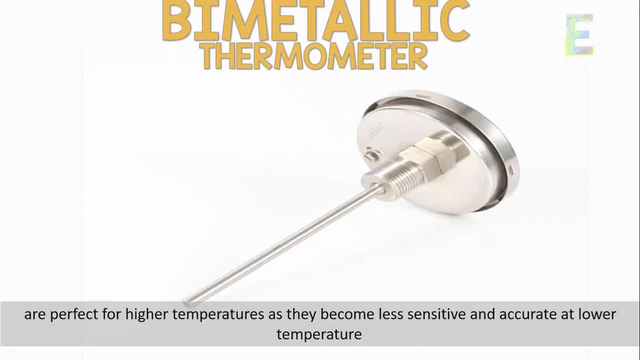 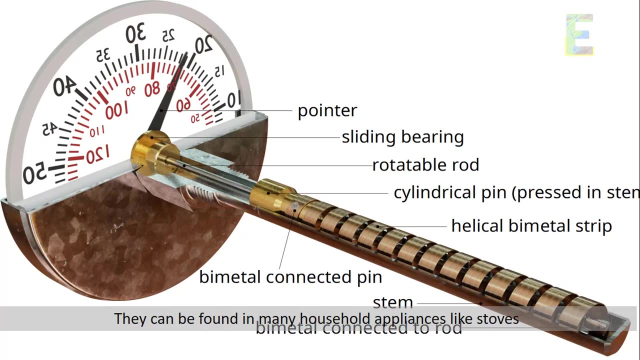 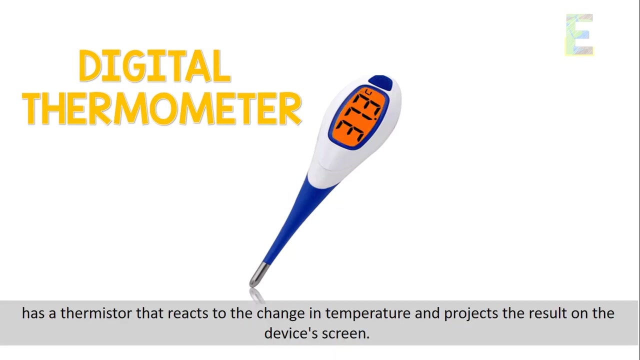 Biometallic thermometers are perfect for higher temperatures, as they become less sensitive and accurate at lower temperature. They can be found in many household appliances like stoves, A digital thermometer. It has a thermistor that reacts to the change in temperature and projects the result on the device's screen. 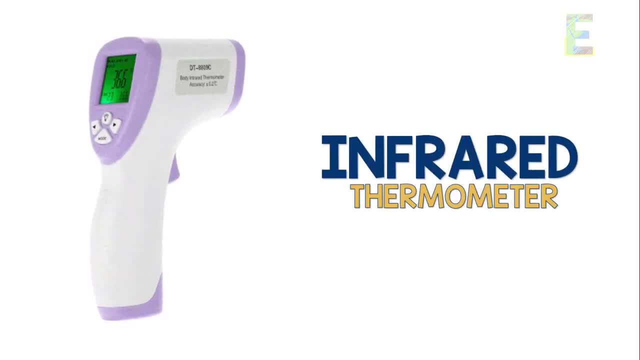 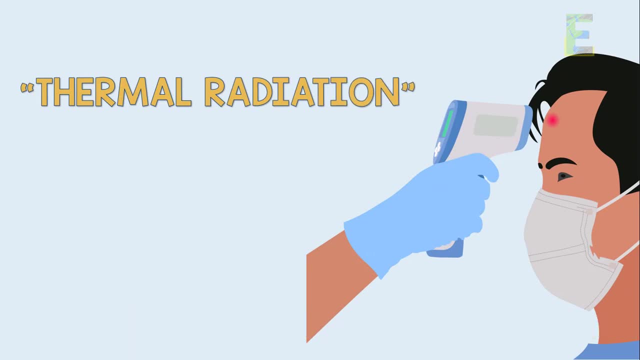 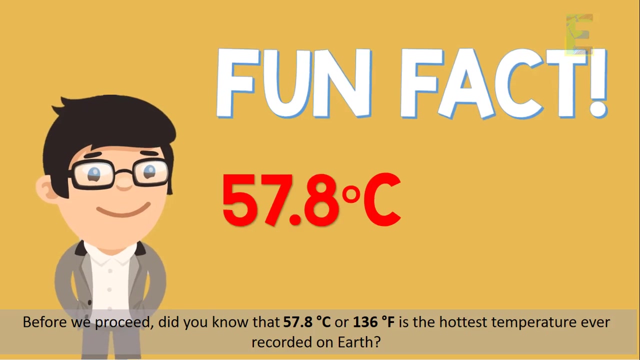 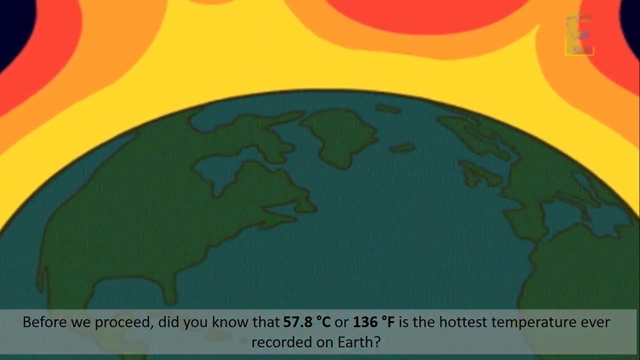 last kind of thermometer is the infrared thermometer. an infrared thermometer uses thermal radiation that objects emit to measure thermometer. now let's have a fun fact before we proceed. did you know that 57.8 degrees Celsius, or 136 degree Fahrenheit, is the hottest temperature ever recorded on earth? it was recorded. 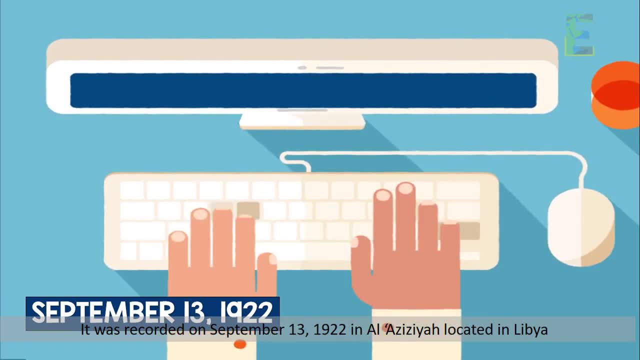 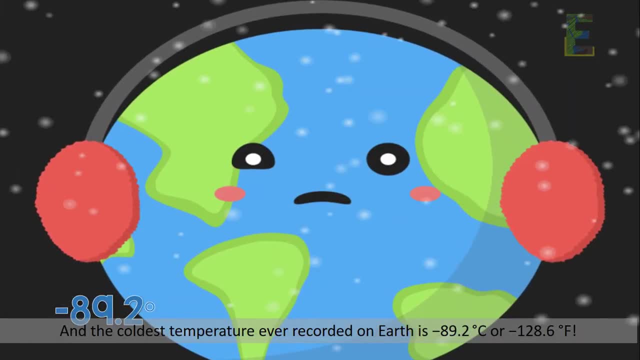 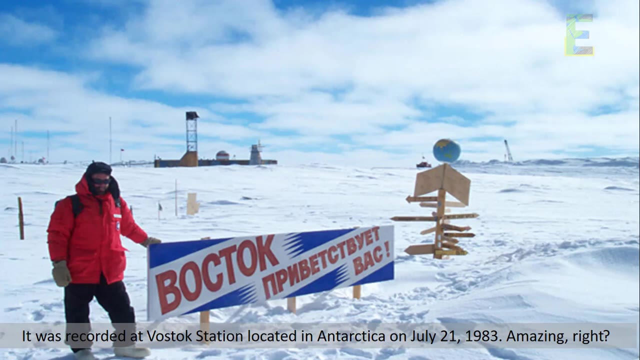 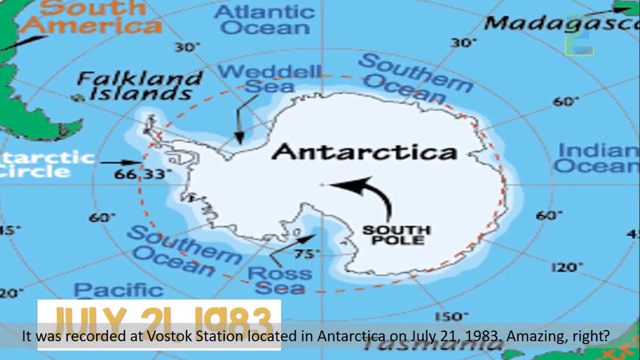 on September 13, 1922 in Al Zazaya, located in Libya, and the coldest temperature ever recorded on earth is negative 89.2 degrees Celsius or negative 128.6 degree Fahrenheit. it was recorded at Vostok station, located in Antarctica, on July 21, 1983- amazing, right now, going back to our topic, temperature. 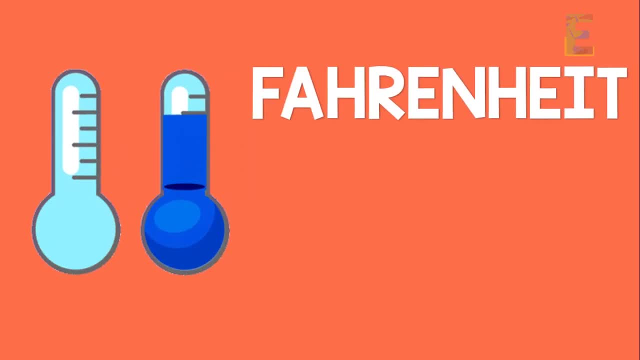 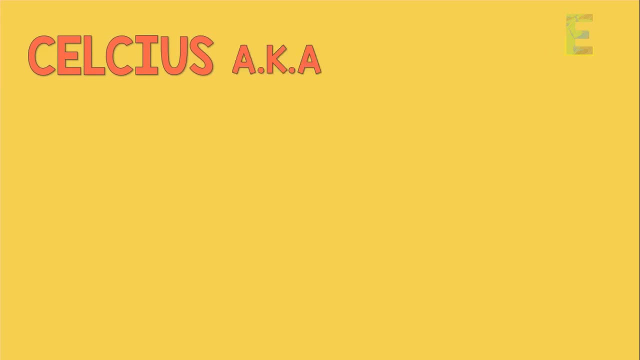 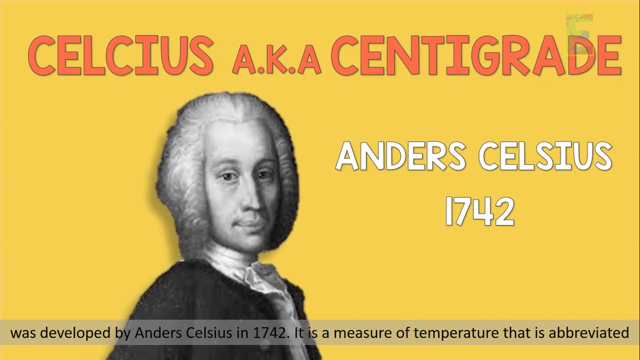 is measured by temperature, and temperature is measured by temperature in many different scales, including Fahrenheit, Celsius and Kelvin. let us tackle them one by one. Celsius, also known as centigrade, was developed by under Celsius in 1742. it is a measure of temperature that is abbreviated by C. 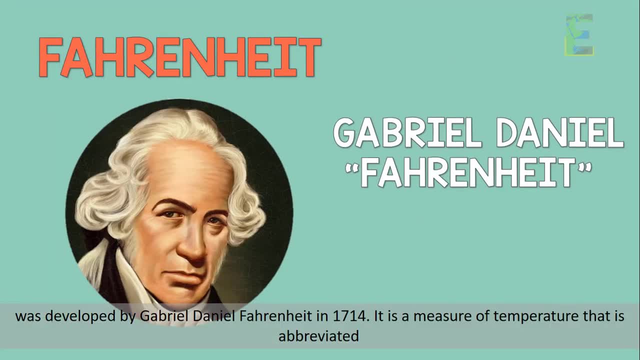 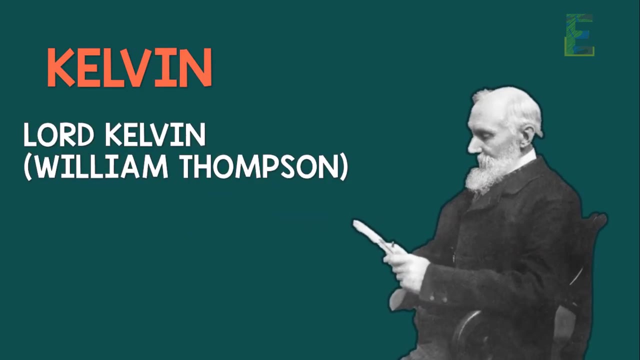 Fahrenheit was developed by Gabriel Daniel Fahrenheit in 1714. it is a measure of temperature that is abbreviated by C, with F Kelvin. this was designed by Lord Kelvin William Thompson. it is a measure of temperature that is abbreviated with the letter K. moreover, Kelvin is a temperature scale designed so that zero Kelvin is defined as absolute zero, and